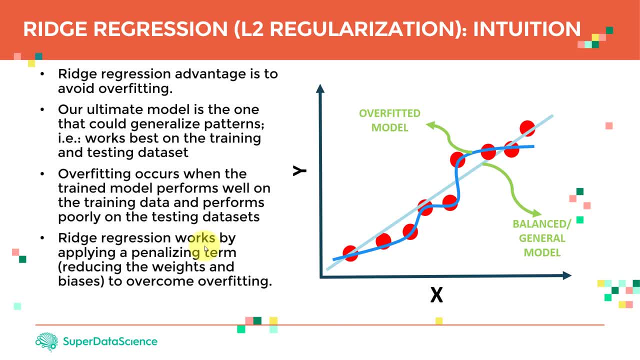 the two models. So we're going to try to reduce the variance between the two models. So we're going to try to reduce the variance between the two models. So we're going to try to reduce the variance or the variability among two data sets by trying to increase the bias a little bit. Okay, I know. 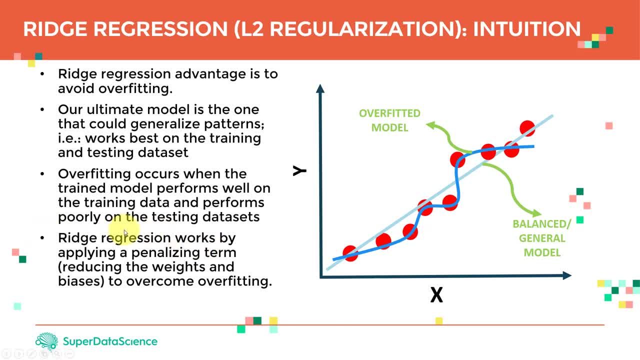 it might sound a little bit confusing, but the overall idea is that we wanted the model to perform maybe a little bit worse during training, but for the sake of the greater good, which is the model will become more general and will become doing well during training and during testing, as 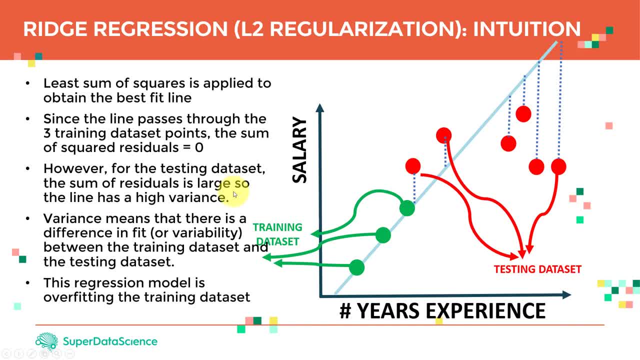 well, All right, let's dig a little bit deeper. So let's assume that we have two models here, this practical example: Let's assume that I have these three green points, green dots and these are the training data. And let's assume that I went out there and we used the least sum of squares. 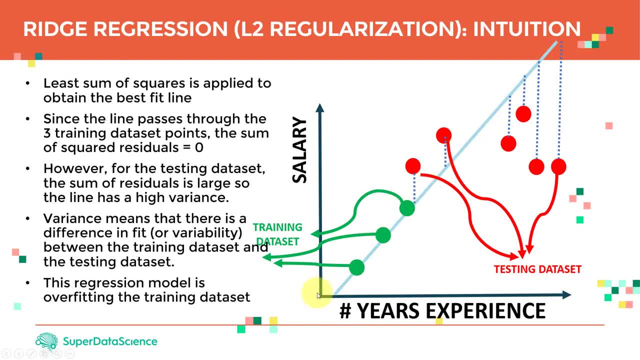 to draw a line that goes through the training data And, as you guys can see, because I only have three dots or three points, I've been able to pass a perfect line in here. Looks good, right, Okay. so, since the line again passes through the three training data, sets the sum of square. 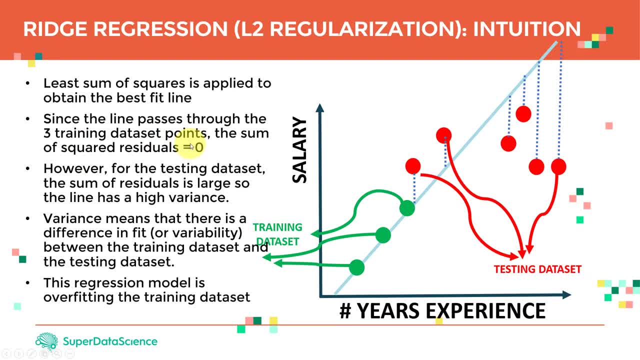 residuals is equal zero, which means that model is perfect during training. However, if we take a little bit, you know, like a greater look at the entire data set, you will find that my testing data set looks very different. So these red dots here, these are the testing data set. So for the 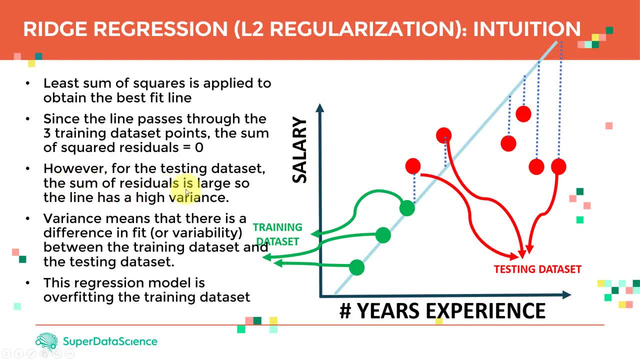 testing data set. the sum of residuals is large, So the line has a high variance, which means that will perform great during training. It actually passes exactly on the training data. However, it performs very poorly on the testing data set And variance means that there is a difference in 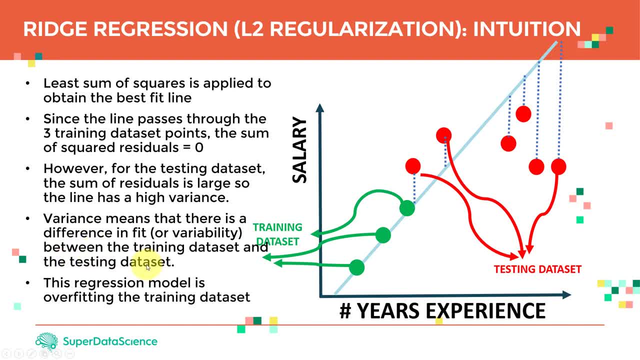 fit or variability between the training data and the testing data, And this regression model we call that. it has overfitted the training data set. All right, Again, we haven't clearly discussed what we mean by ridge regression. So that's happening right now. So what ridge? 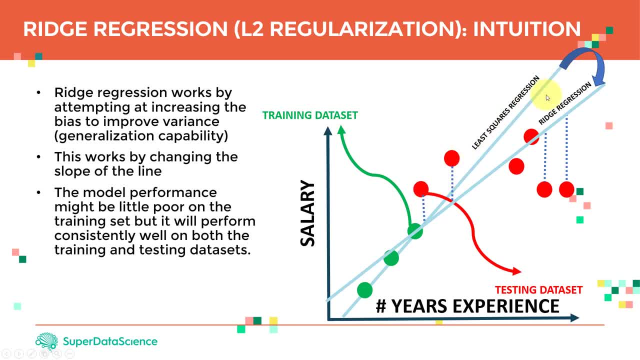 regression we're going to do? we're going to say: you know what, let's take that line and maybe shift it a little bit, just tilted or rotated a little bit, as you guys can see here. So when we rotate it a little bit, 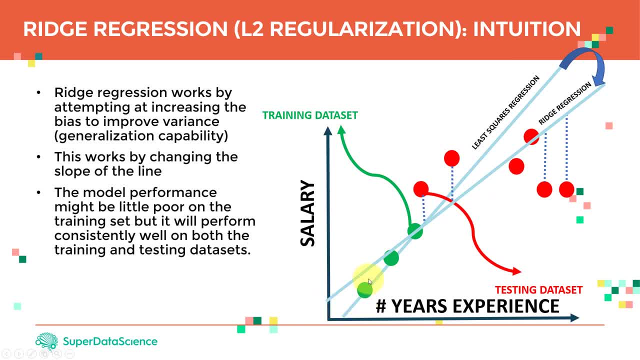 yes, we're going to introduce a little bit of additional error during training because the line now does not go through the three data points. However, the model will perform better during testing. Okay, It will actually become more general. It will generalize during training. 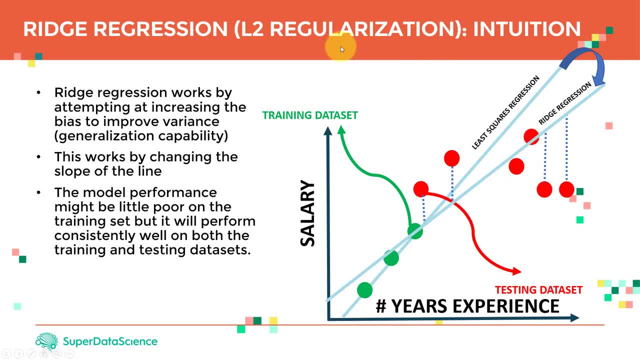 and testing, And that's the overall idea of regularization. That's all what it is. So ridge regression works by attempting and increasing the bias to improve the variance or to improve the generalization capability. So this works by changing the slope of the line. So we took that line which is the least square. 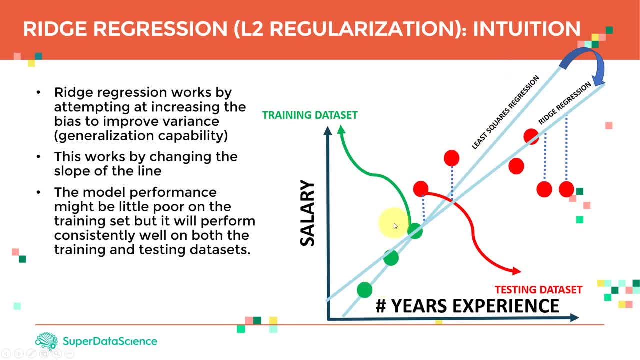 regression line and then we shifted a little bit. We're just going to tilt it and that will be my ridge regression line. The model performance might be a little poor on the training data but it will improve the generalization capability. So we took that line which is the least square. 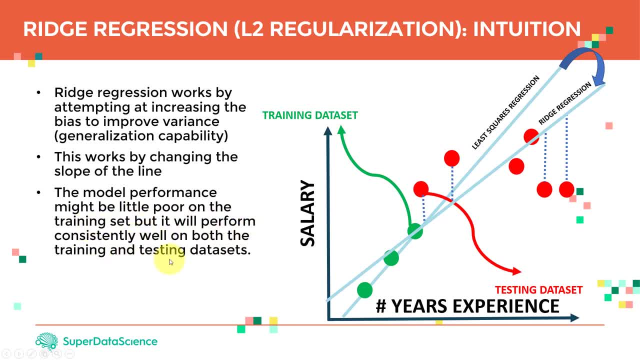 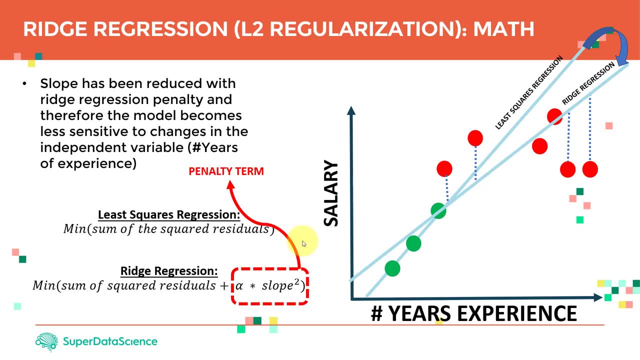 regression line. The model performance might be a little poor on the training data, but it will perform consistently well on both the training and testing data set. That's the overall idea, All right, So let's take a look at some mathematics. So, as you guys can see here, 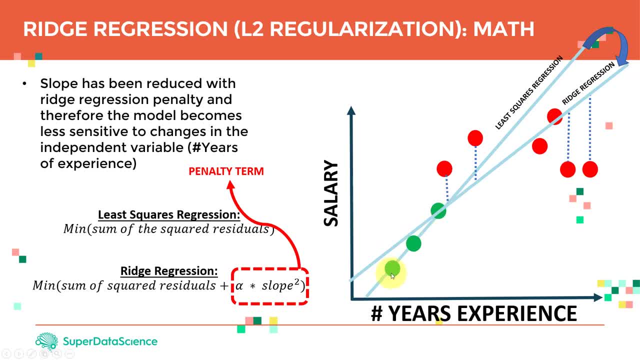 this is simply our least square regression line, which is perfectly matching and going through the training data And, as you guys recall from previous slide, that all these data points are the testing data points and the least square perform horrible on them. So what ridge regression is going to do is that we're going to change the slope of the line. 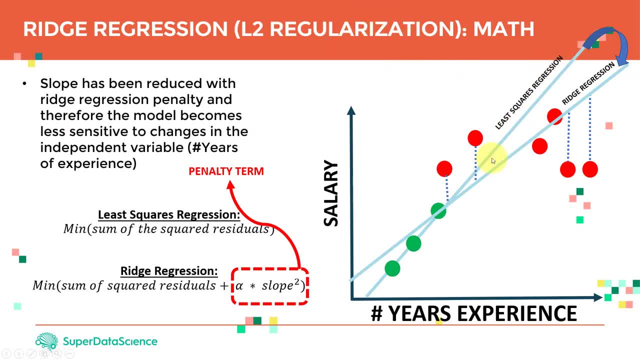 So we're going to tilt that line from here and tilt it a little bit, And that's what the idea of regularization is. So the slope has been reduced with ridge regression penalty and therefore the model becomes less sensitive to changes in the independent variable, which is 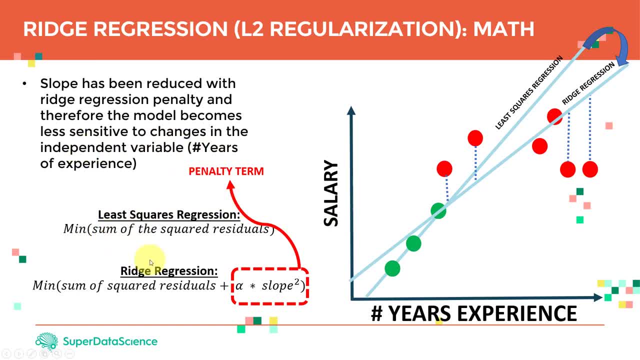 number of years of experience. What do you mean by that? So if we try to compare basically the two techniques, so you find that least square regression, we're going to try to minimize the sum of the squared residuals, which is simply the error between the points, between the data points and the actual. 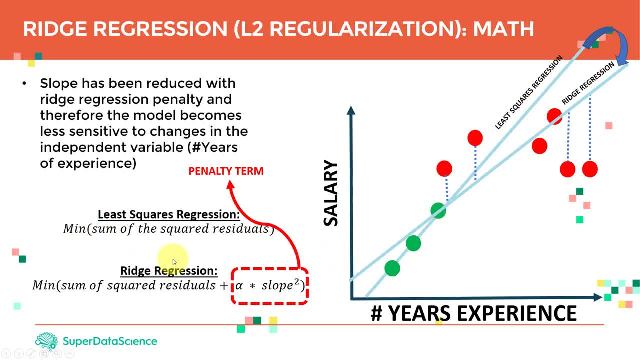 fit or actual line. What ridge regression we're going to do? we're going to try to minimize the sum of square residual, but we're going to add an additional penalty term which is going to be alpha times slope squared. That's all what it is. So that's the overall idea of ridge regression.